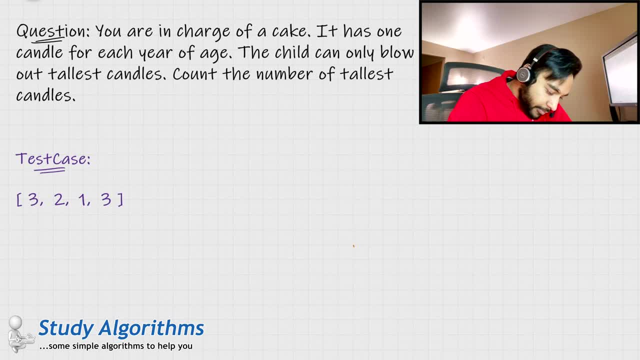 so in this problem, you are given a cake and on this k, let us say, you have some candles. so in a test case you have candles of the height 3, 2, 1 and 3, so they could be something on the cake like: this is your test case: you have a cake and on the cake you have candles of different. 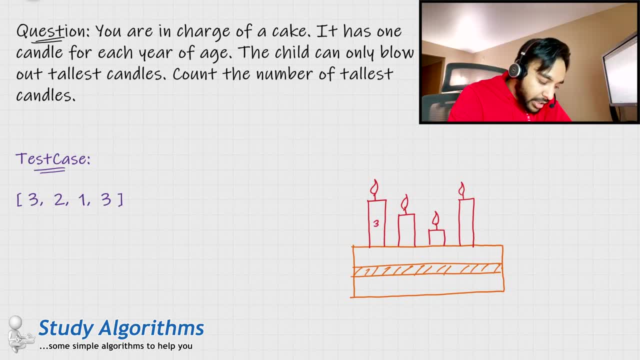 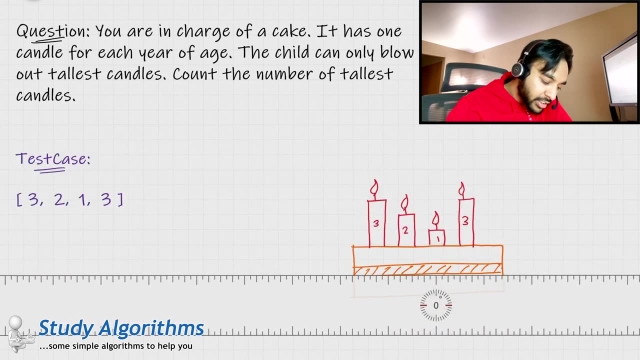 lengths. one is of the length three, then two, then one and then three again. and, as per the question, when a child blows the candles, only the tallest candles gets blowed out. so if you look at this cake, which one is the tallest candle? you start from the bottom and then you go up. 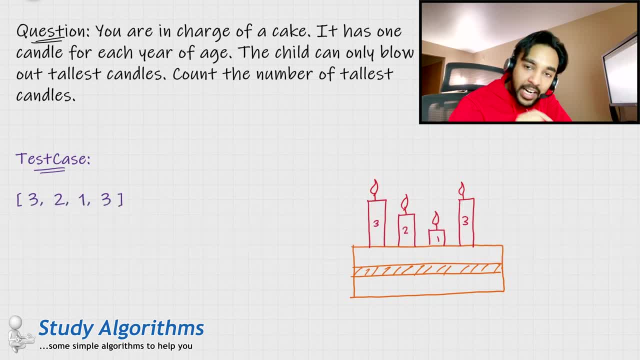 you see that no candle is larger than the candle number three and hence, when you will blow out, these two candles will get blown out and hence, in this case, your answer would be two. so all you need to do is given a cake and some height of candles. you need to find out the tallest. 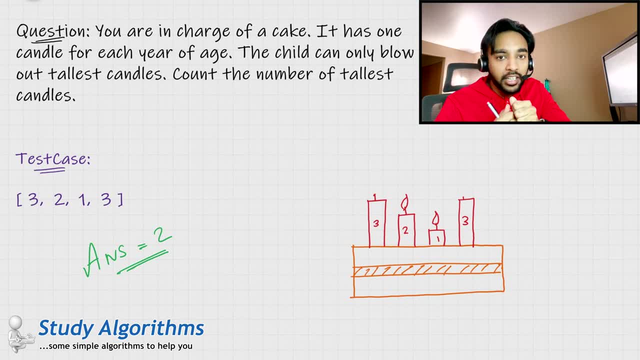 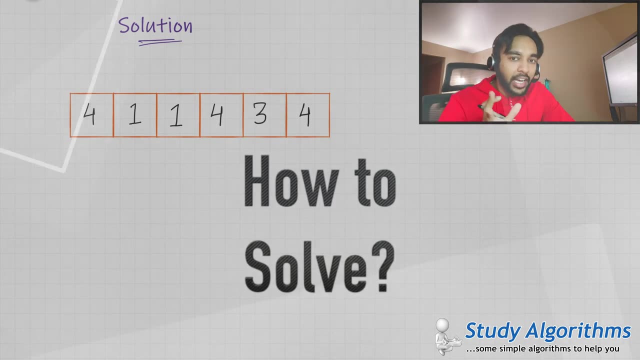 candles and find out how many tallest candles are there, and that would be your answer. if this problem is now clear to you, you can feel free to try it out on your own. otherwise, let us see how we can solve it. let us suppose that the heights of the candles that you are given are in an array like this: 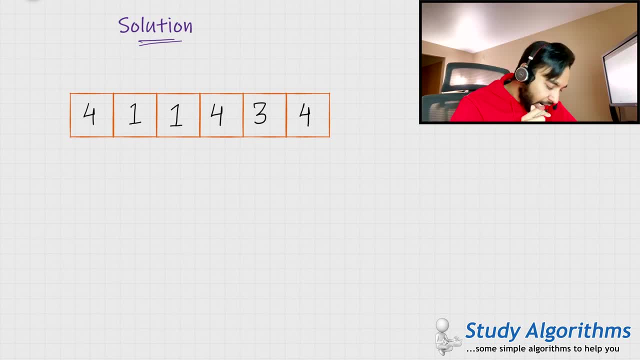 so these numbers represent the heights of the candles. what they simply mean is you have candles like this height 4, 1, 1, 4, 3 and then 4 again. so how you can solve it, what you can do is you can start from the first position in the area. 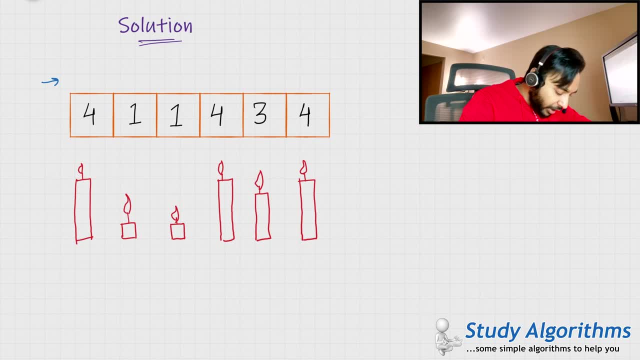 and then keep a track of what is the tallest height that you can find so you can have a value maxim and this will store the length of the tallest candle. so you start iterating from the first position and linearly you pass throughout the entire array. so if you do a complete scan of the area, you would see. 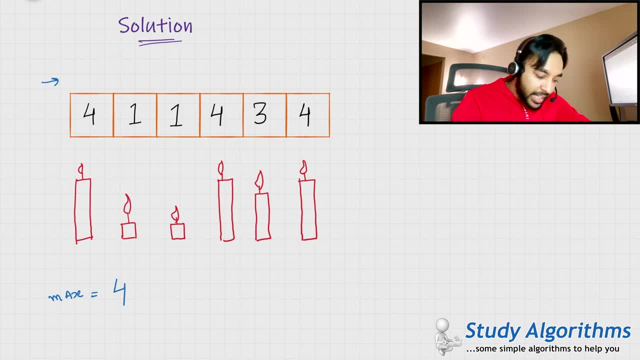 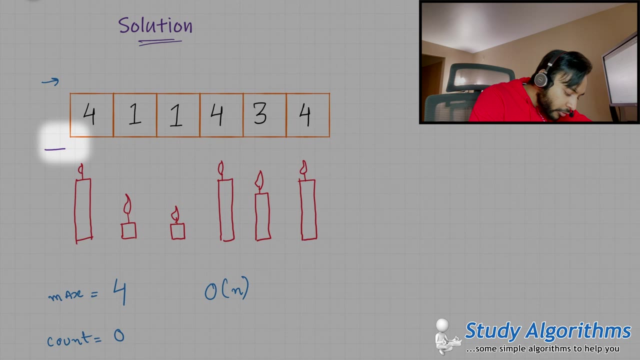 maximum value you can find out is four, and that takes an order of n time. right, This is the length of the tallest candle right In the next iteration. what you simply do is you keep a value count and that is set to zero. I trading over the array for the 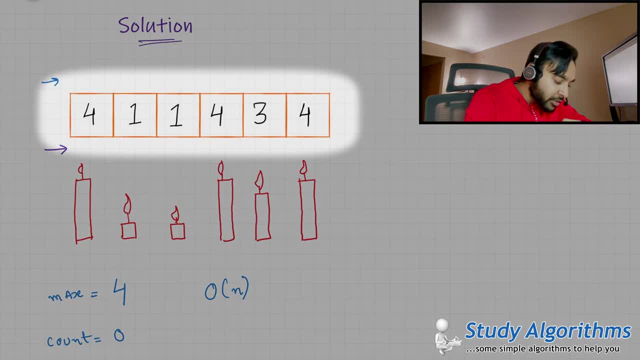 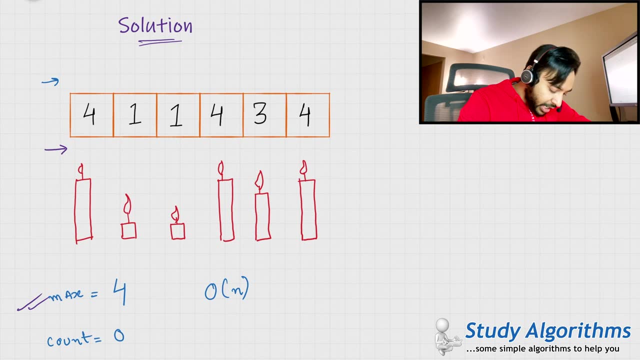 next time. What you now do is you compare each of the values in the array to your maximum value. So you see that four equals the maximum value, correct? So increment the count by one. Next one does not equal four, So this is not the tallest candle. Once again, one. 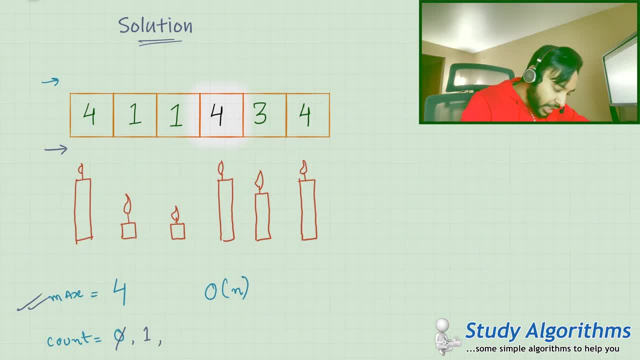 is not equal to four. Going ahead, you see four again. So this time you would again increment the value of count to two. Moving ahead, you see the value three. It is not equal to four, So you don't do anything. Moving ahead, you see the value four. 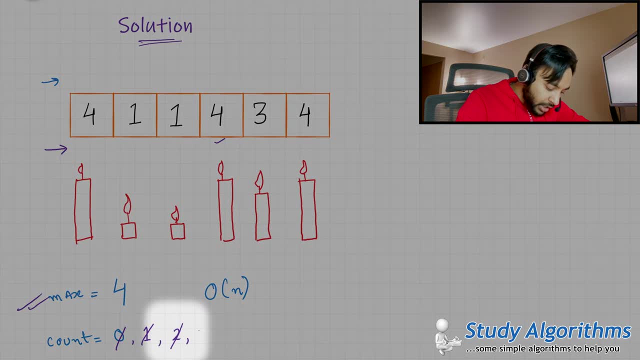 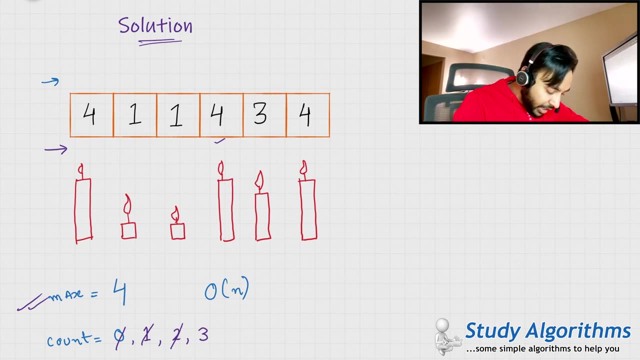 This is again equal to the maximum value. So you increment the count by one As soon as you reach the end of the array. that's it, You have arrived at your solution, and the value of count will store your answer. So if you blow out the candles, then three. 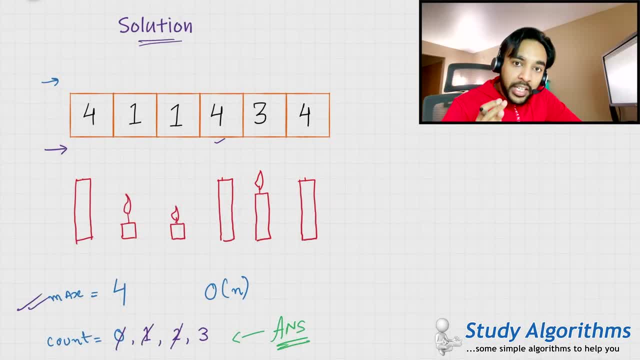 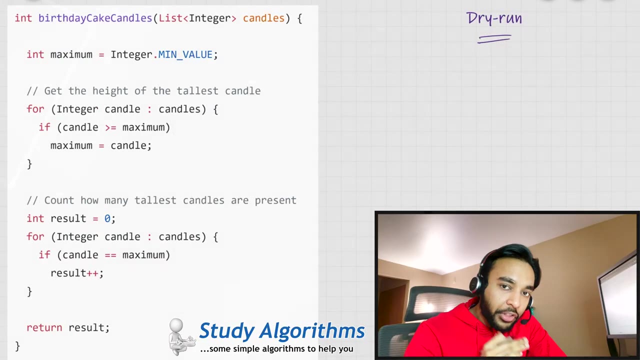 candles would be blown out right Now. this solution works in an order of n time complexity. That is because we scan through almost all of the elements of the array linearly. Now let us do a dry run of the code and see how it works On the left side of your screen. 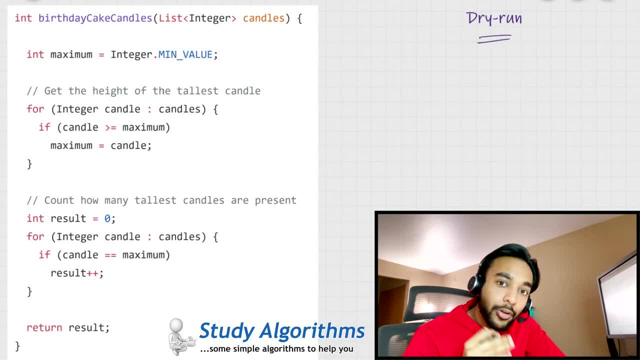 you have the actual code to implement this solution. And on the right, let us take up an example. Let us say we have the candles of length. So this is a list of candles and it is passed in as a parameter to our original function. Next, what we do is we keep a variable. 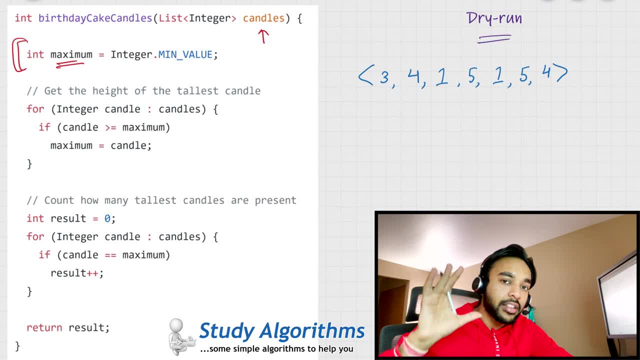 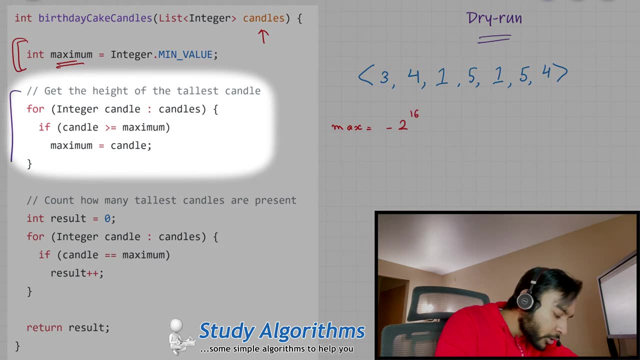 maximum. This is the length of the maximum candle that we can find in a list. So right now, the value of max is assigned to a very small value, That is, minus two to the power of 16.. Next, what you're going to do is you are going to get the height of the tallest candle. What 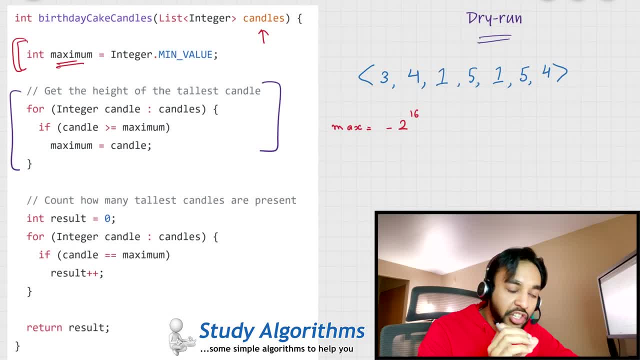 you do is you compare the value max with each of the values in the list. So if the value in the list is greater than the maximum value that you have, that means that is a taller candle, right? So right now, the value of max is minus two to the power of 16. And you? 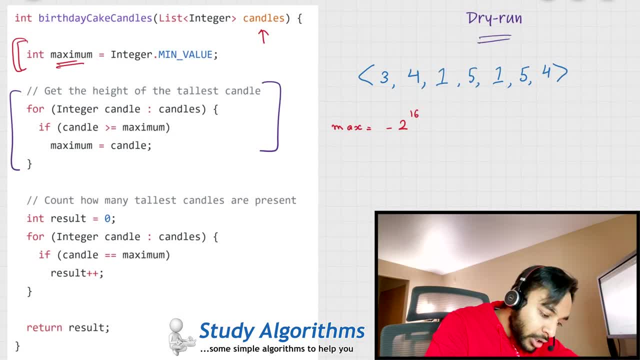 compare it with three, Since three is larger, so this would change to three Going ahead. you compare the value maximum with four, Since four is larger, this changes to four Going ahead. you compare this value with one: One is smaller, so you don't update it Going. 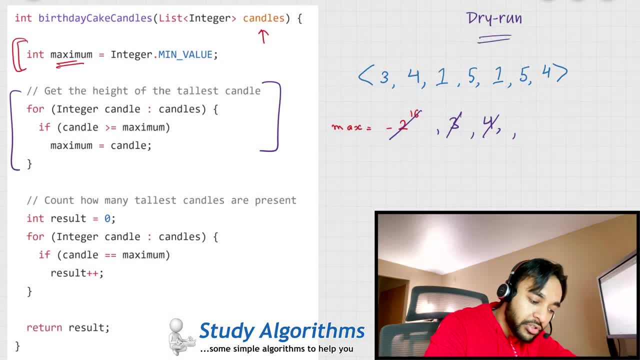 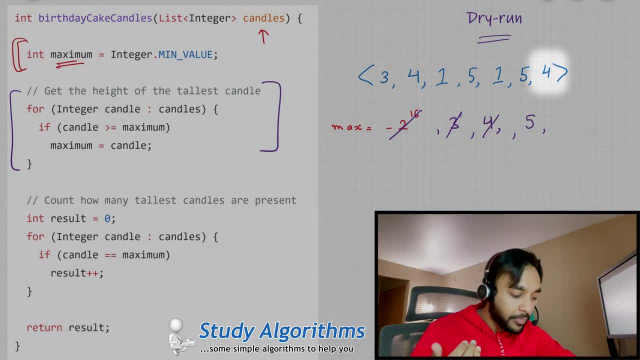 ahead, you compare this with five. Since five is larger, you change it to five. Going ahead, you see the value, one which is smaller, Five is again equal and four is smaller. So up till now, you find out the maximum value and that comes out to be five. 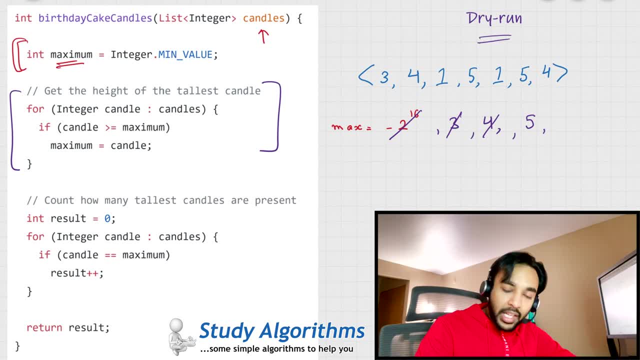 That means five is the length of the tallest candle. Now it's just a case of finding out the count of this tallest candle. So what you do is you keep a value result and this would store the count of the tallest candles. You again start iterating towards your entire list And you compare if five is equal to 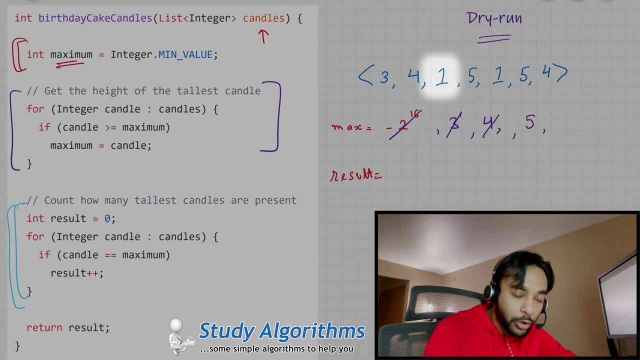 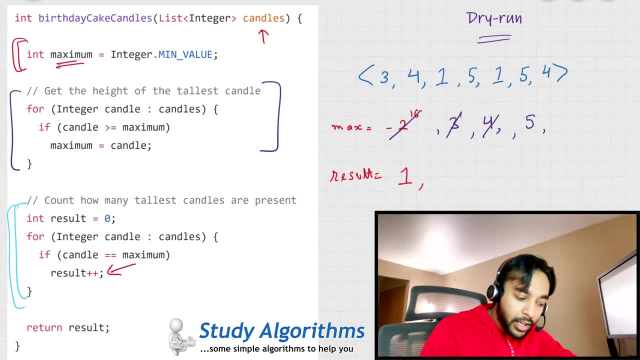 three: no. If five equal to four, no. If five equal to one: no, Five is equal to five. So you increase the result by one. Going ahead, you see one again, So you don't do anything. Next, you see five. So once again, you increase this value and the value of result changes. 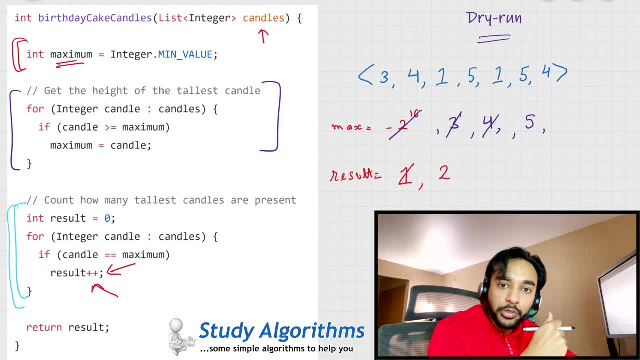 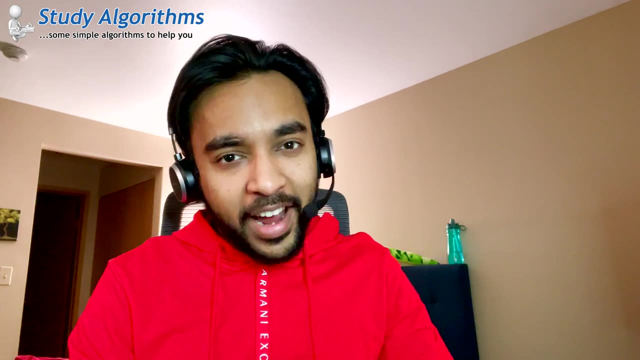 to two. Now this loop ends because you have iterated towards the entire list And the value list would contain your answer. I hope I was able to simplify the problem and its solution for you. Go ahead and solve this problem on HackerRank now. As per my final thoughts, I want to leave with an idea. 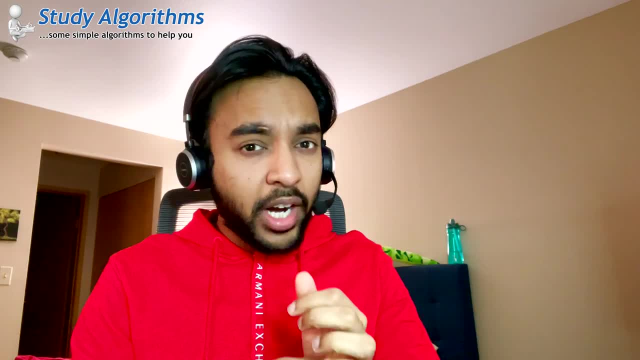 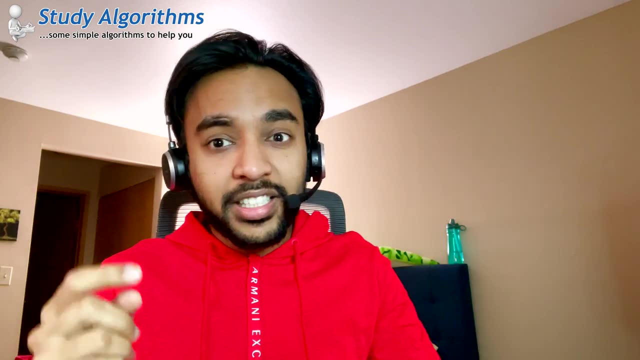 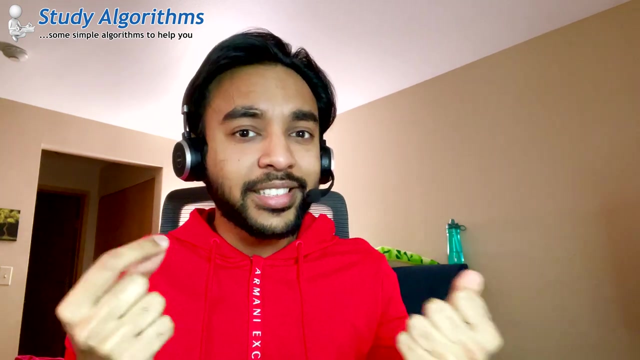 in your mind. The solution we just discussed required two iterations of the array, right. Could there be a way that you could count the number of maximum candles just in a single iteration? You have a stream of numbers and you want to find the occurrences of the maximum number.